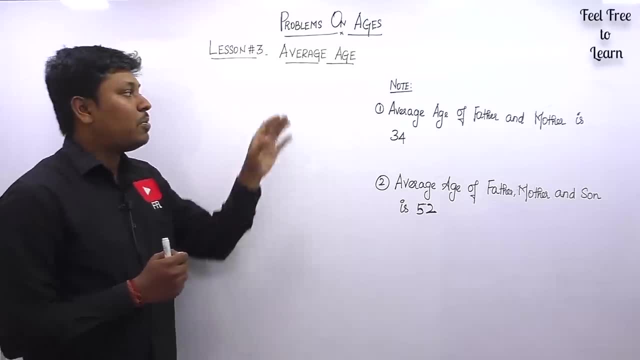 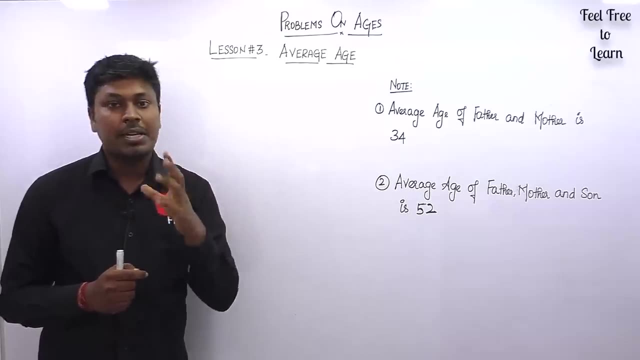 all the five questions, you need to know little bit basics about the topic. average, What is called as average Average, is equal to sum of observation divided by total number of observation, which we have seen in many videos. I think I have posted seven different lessons. 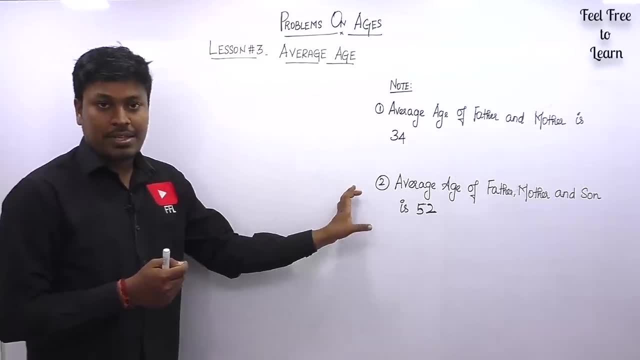 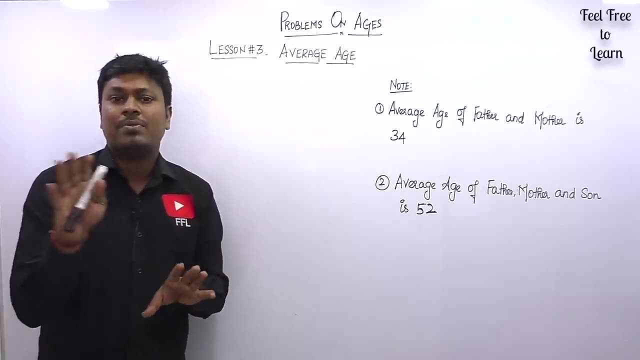 on the topic average. So for solving all the questions that is based on average, you need to know little bit knowledge about average. That is more than enough. Just a formula is enough. What is formula for average? Just now I have told you: sum of observation divided. 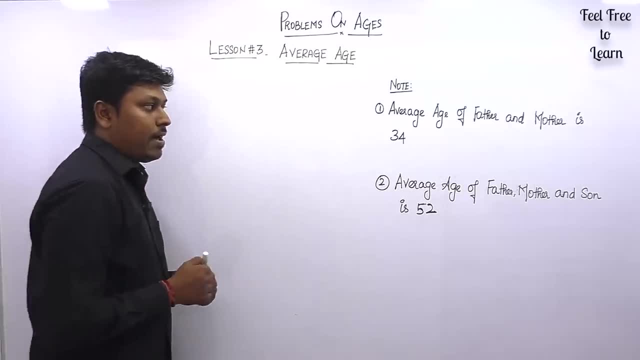 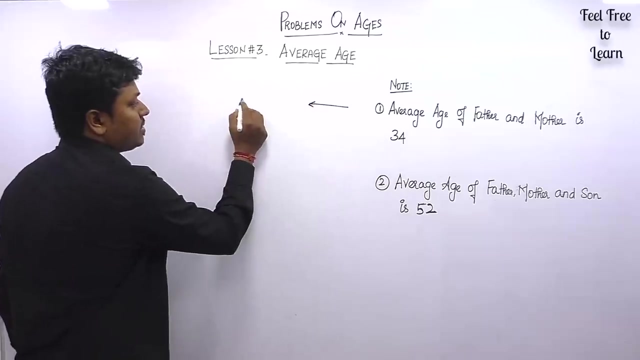 by total number of observation. So note number one: average age of five years, father and mother, is 34.. What is the meaning of it? Average age of two person: one is father and the second person is mother. Their average is 34.. So this can be written as sum of observation. 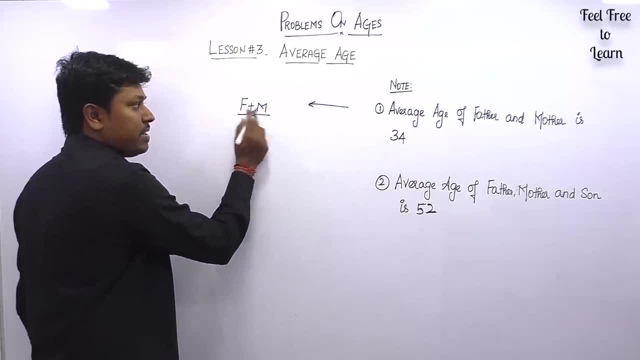 So father and mother average total number of observation. There are two person, So divided by two is equal to 34.. So average age of father and mother is 34.. So we can say that father and mother 34 into two will be 68.. 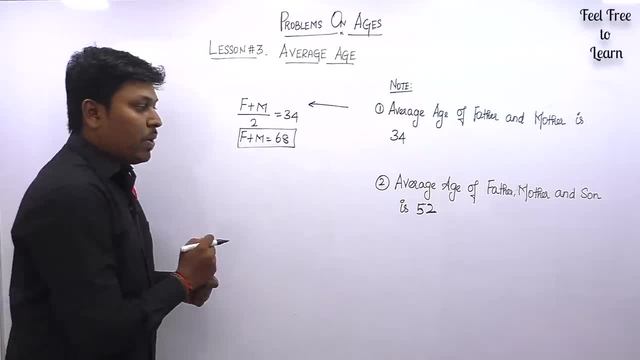 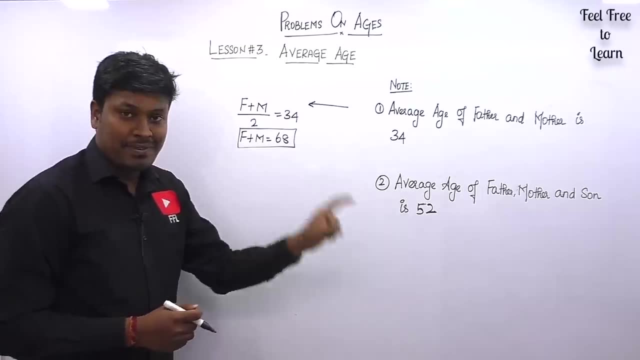 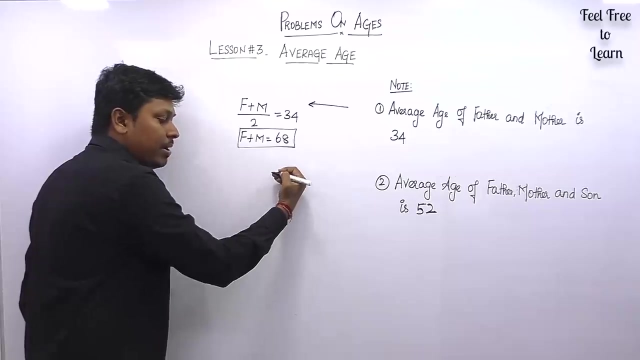 It is just a basic. So point number two: average age of father, mother and son is 52.. So average age of three person: father, mother and a son. So average is equal to sum of observation divided by total number of observation. In the numerator sum of observation there are: 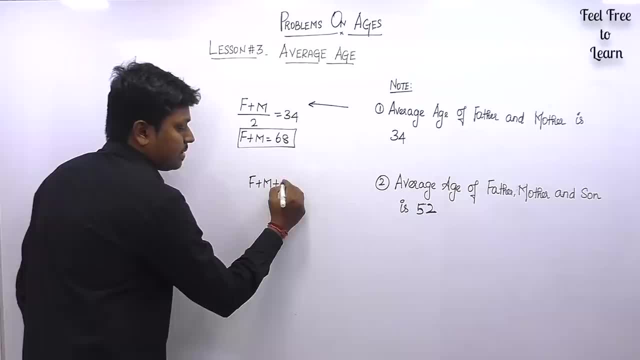 three person: father, mother and a son. divided by total number of observation, There are three person. So it's divided by three is equals to 52. So father, mother and son is equals to 156.. So sum of their ages will be 156. If they are. 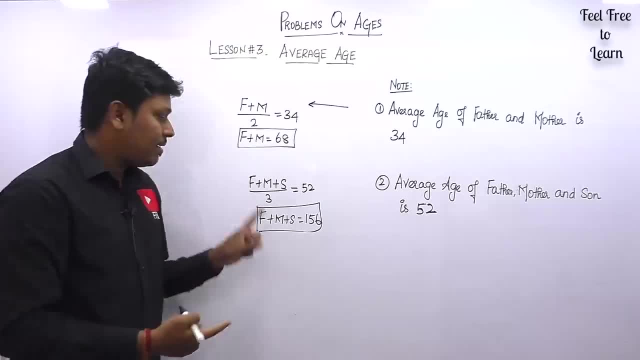 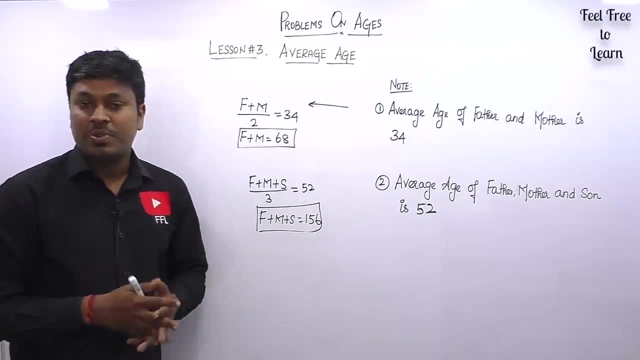 talking about four person divided by four. if they're talking about six person divided by six right. Just a basics. So this is enough to solve a question that is based, on average, on problems on ages. So let me move on to all the five questions Now. question number: 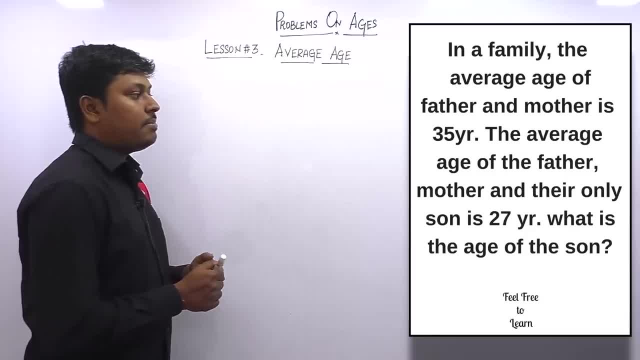 one in a family, average age a father and mother is 35 years. The average age of father, mother and the only son is 27 years. What is the age of the son? So really easiest question. I think we have solved many questions based upon this pattern in the topic average right, Just. 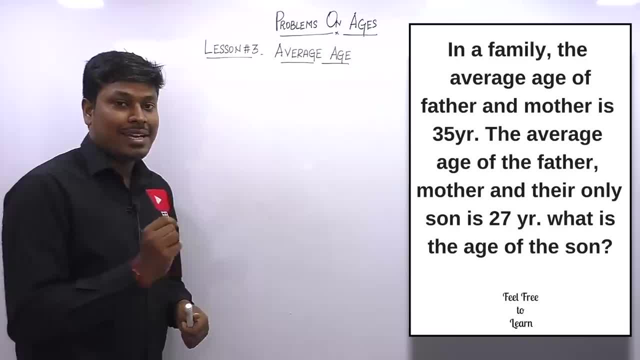 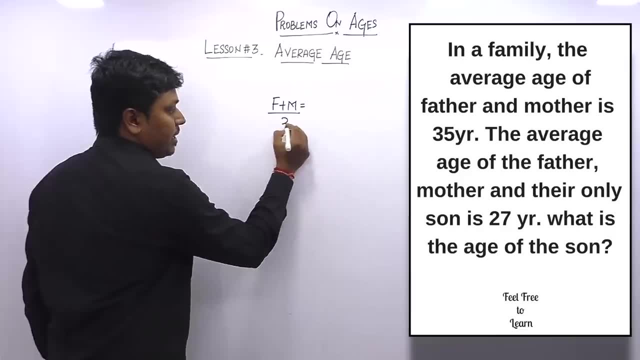 a basic question, right? First, what they are saying is: in a family, the average age of mother and the father. there are two persons, So father and the mother. average age so divided by 2 is 35.. And then the second point: average age of father, mother and the only son. so totally we. 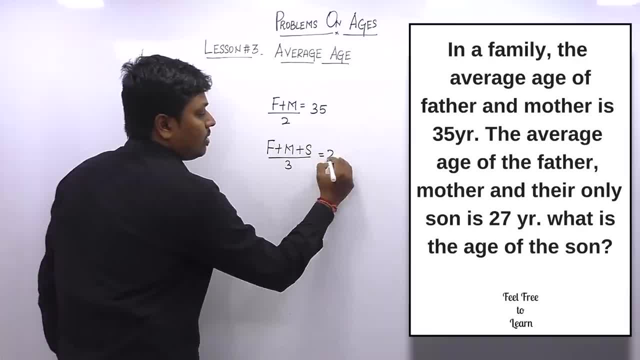 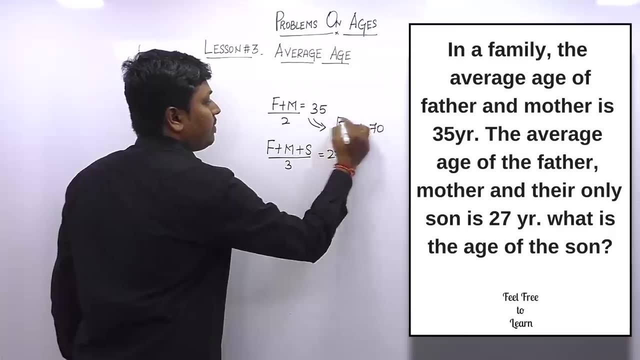 have 3 persons. so divided by 3 is equals to how many years? 27 years. So now our target. to find what is the age of the son. It is really easy, because we know father and mother average age is 35. So we can say that the total age of father and mother will be 70. So 35 into 2 will be 70.. 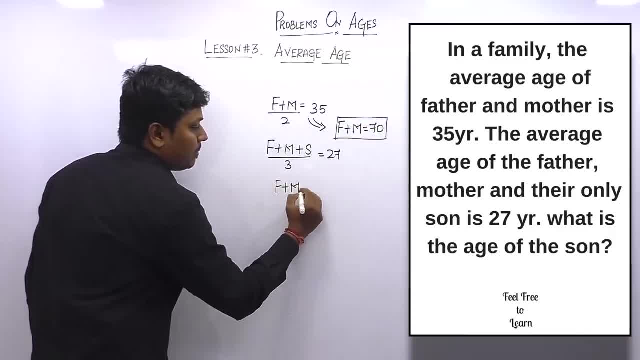 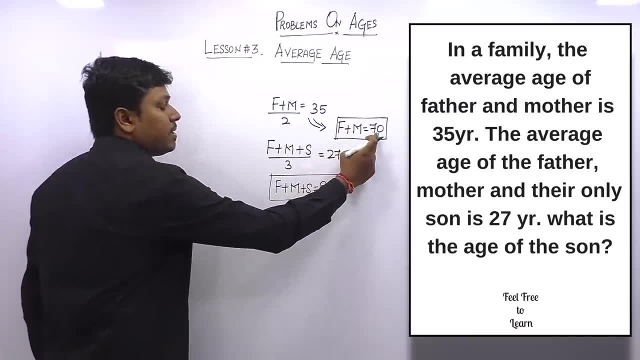 So according to the second equation, total age of father, mother and the son is equal to 27 into 3 will be 81. And we already know father and mother total age will be 70. So instead of father and mother substitute here, 70 plus S is equal to 81. 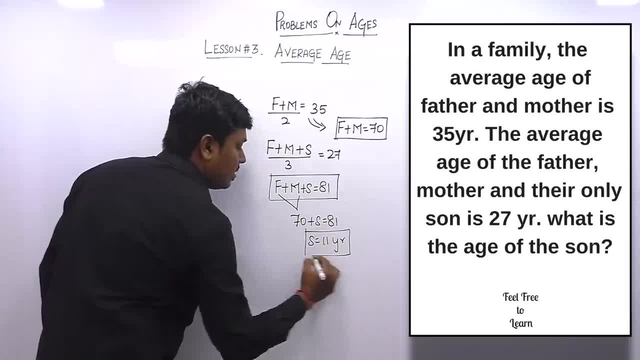 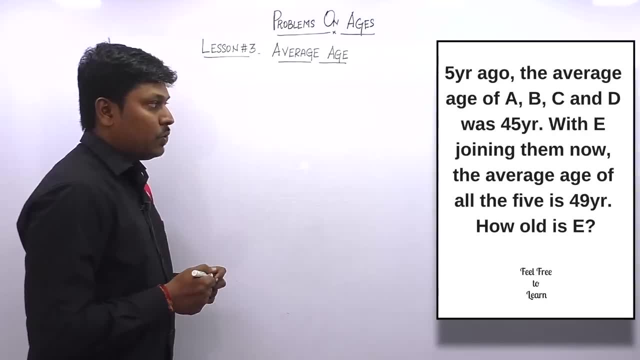 So S is equal to 11 years. It is really easiest equation. So finally, for the first equation, the age of son is 11 years. Question number 2.. 5 years ago, the average age of A, B, C and D: 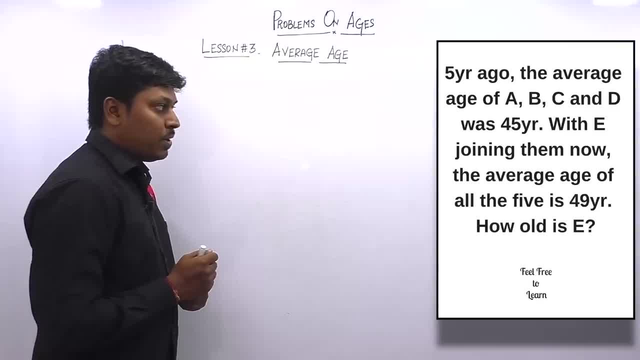 was 45 years With E joining them. now the average age of all the 5 is 49 years. How old E is? So listen to the question. First point: they are talking about past because 5 years ago. In the next point, E joining them now. 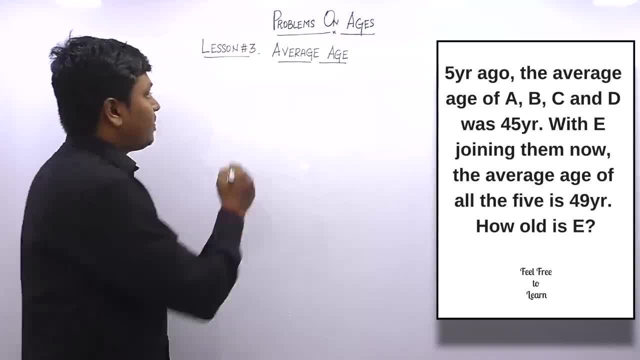 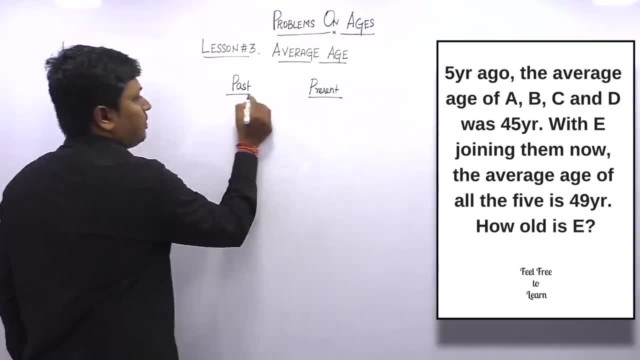 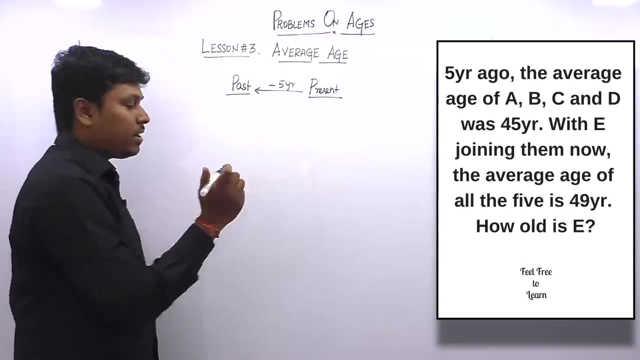 So in the second point they are talking about the present. Got it? So first point, they are talking about past, And the second point they are talking about present And from the present to the past. 5 years ago, So 5 years ago, average age of 4 person is 45.. 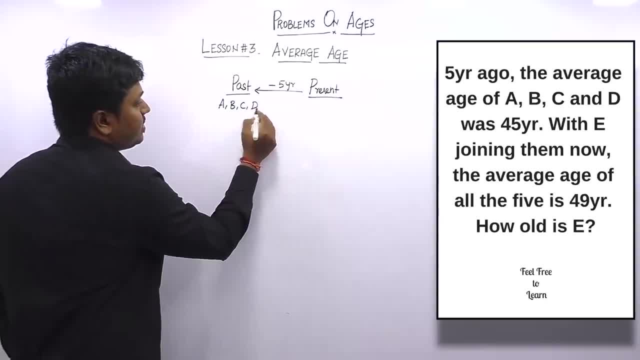 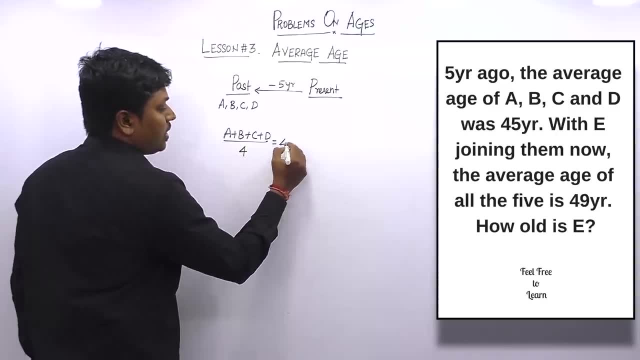 So we can say A, B, C and D. So 5 years ago, average age of 4 person So divided by 4 is equals to 45. So we can say A plus B, plus C plus D. 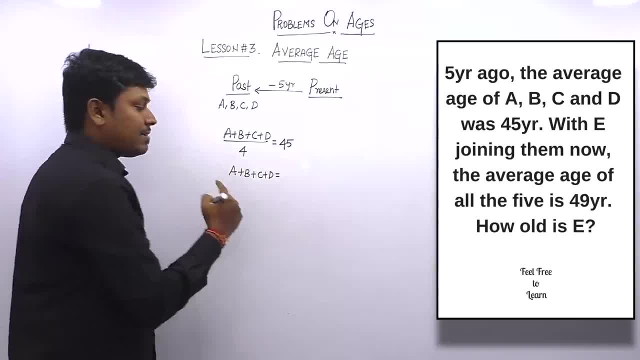 So 4 person sum of their ages 5 years ago will be 45 into 4.. So 4, 4 is 16,, 20,, 180.. So 4, sorry- 5 years ago, sum of their ages, that is, sum of the 4 person ages, will be 180. 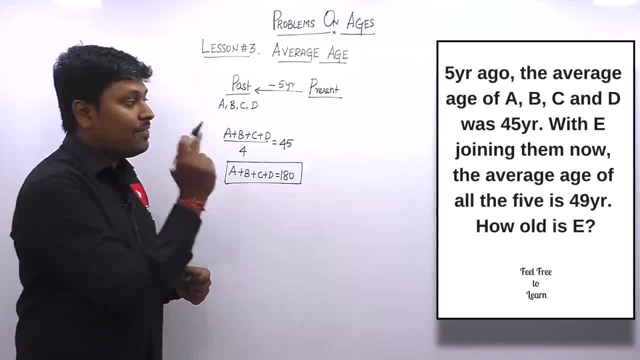 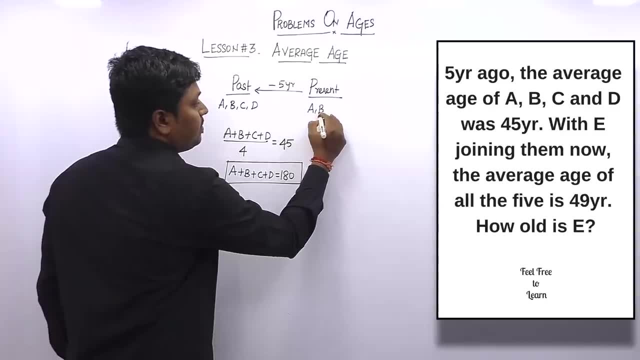 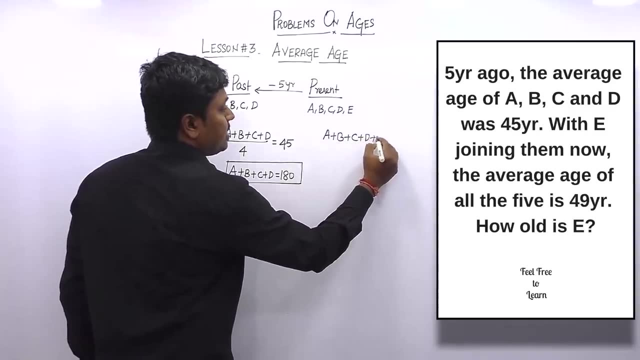 And in the second point now they are talking about the present, With E joining them. now the average age becomes 49. So if E is joining, then A, B, C, D, E, There are 5 person. So we can say A plus B plus C plus D plus E. So 5 person divided by 5 is equals to 49. 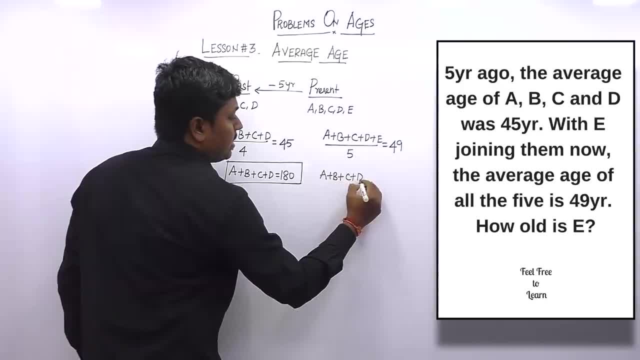 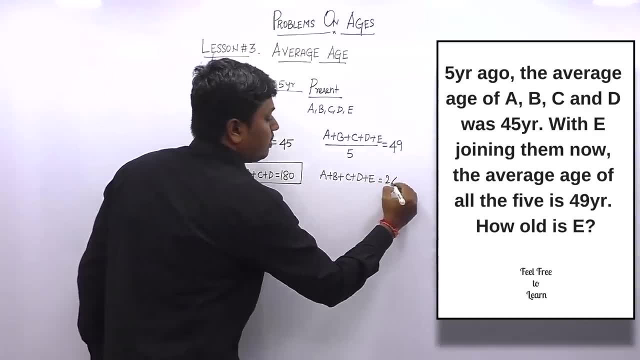 So sum of the ages of all the 5 person D plus E is equals to 5, 4's are 20, 200, 9, 5's are 45, 200 plus 45 will be 245. 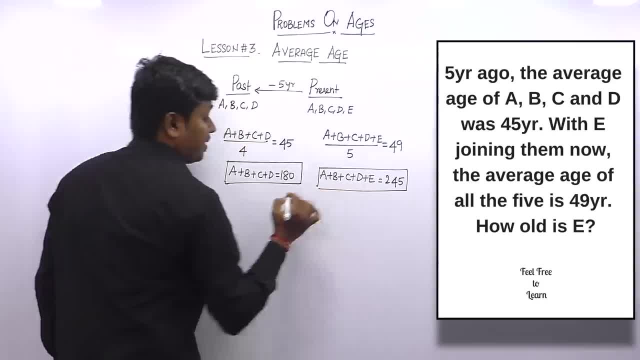 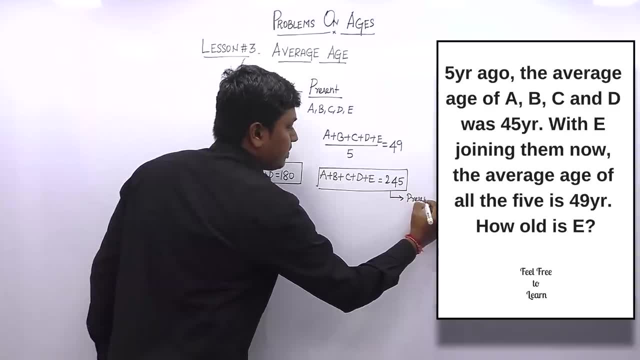 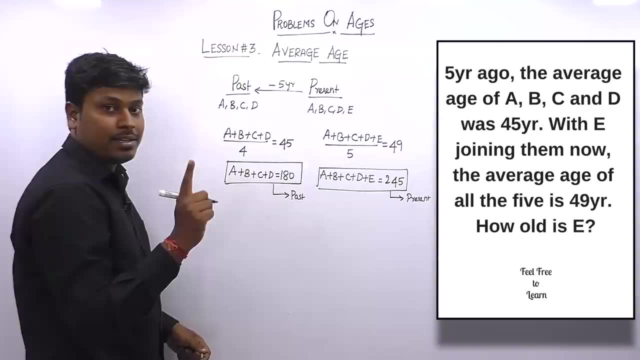 So listen here: sum of the present age of all the 5 person is 245,. right Here it is present And here 4 person sum age that is 180, which is past. We should not directly subtract this. that is wrong. 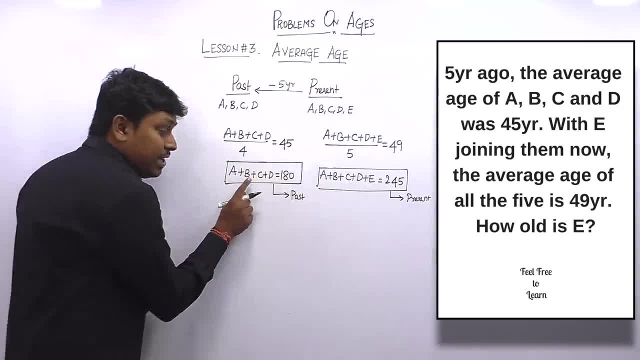 Because this equation we have framed for present And this equation that we have framed is for the past. So let me do one thing. I am just going to convert this equation to the present right. We already know that 5 years back, the total age will be 180. 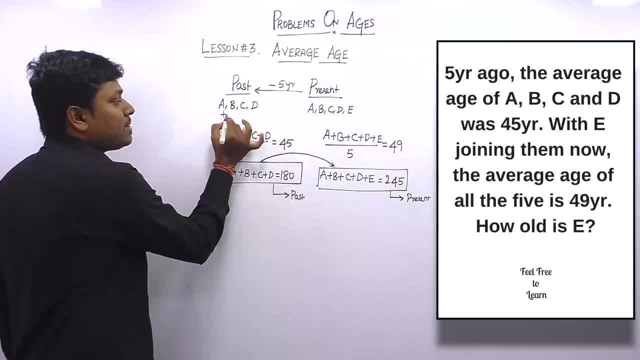 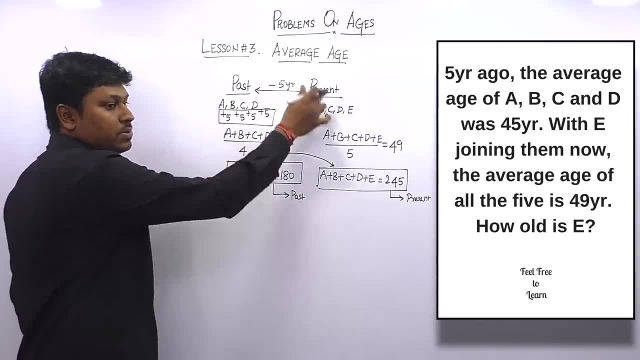 So from the past to the present, for every person, age will be increased by 5.. So 5, 5 and 5. So totally for all the person from the past to the present, the total age 20 will be increased. 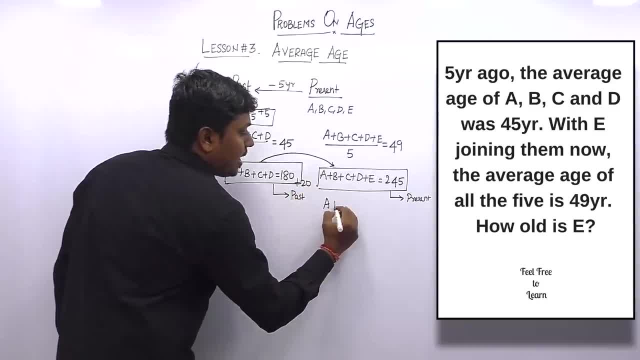 So plus 20.. So now we can say that the sum of their ages, that is, present age of all the 4 person will be 200.. So this equation now we have framed for present. So friends got it. 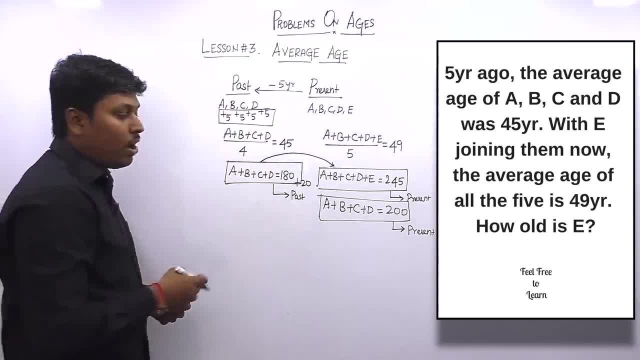 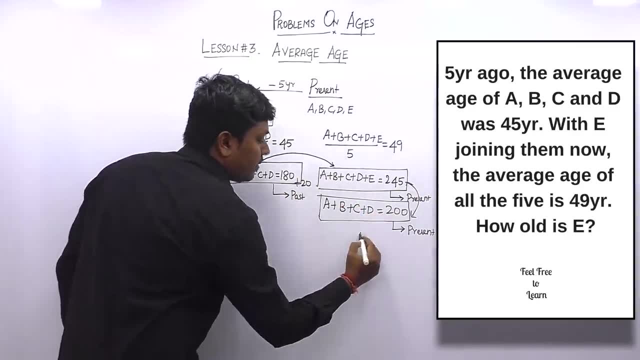 Now we can easily subtract both the equations Because our target to find how old the person E is. So you can directly subtract first and second equation, So that once you subtract 200 and 245, the age of the person E is 45 years. 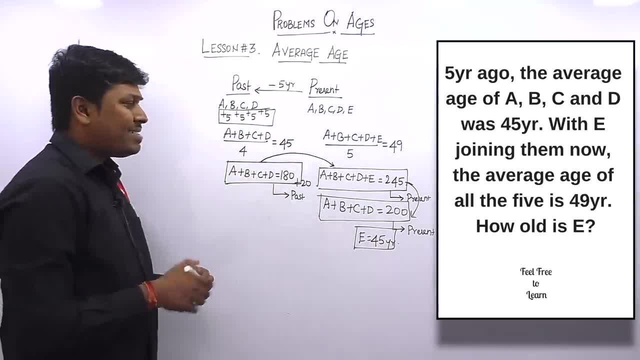 So answer for question number 2 is 45.. And the major mistake of many student is, after writing these 2 equations, they will directly subtract it. No, it is completely wrong. Why? Because the equation that we framed here They are talking about the present. 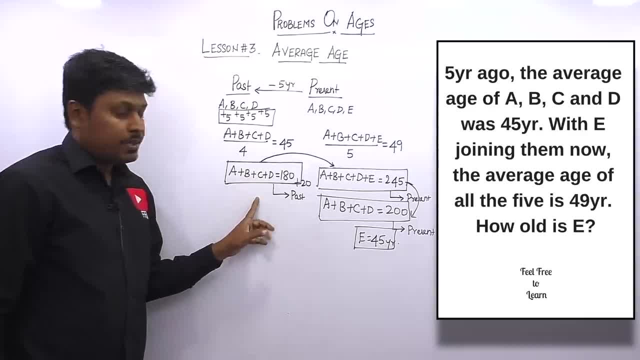 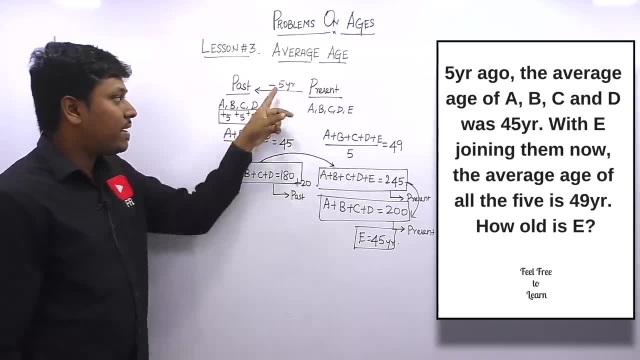 But the second equation that we framed. they are talking about the past, So we need to convert this equation to the present. So, from the past to the present, we already know that the ages will be increased 5 years. So first person A age is increased by 5.. 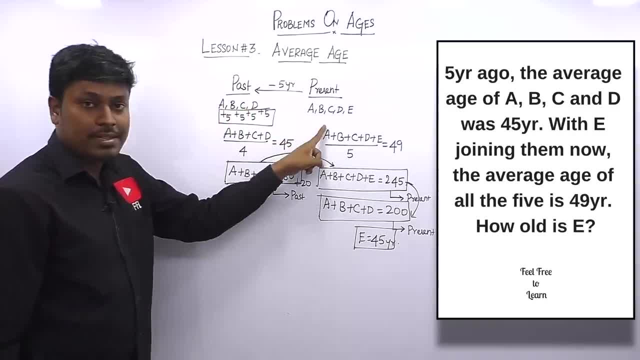 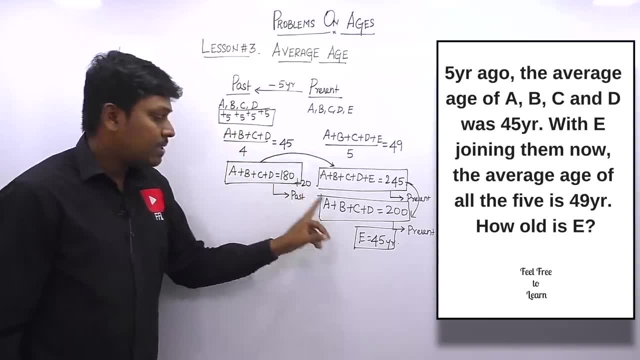 Second person increased by 5, third person increased by 5, fourth person increased by 5.. So totally all the 4 person, the total age increased by 20.. So we can say 180 plus 20, sum of their present age of all the 4 person will be 200. 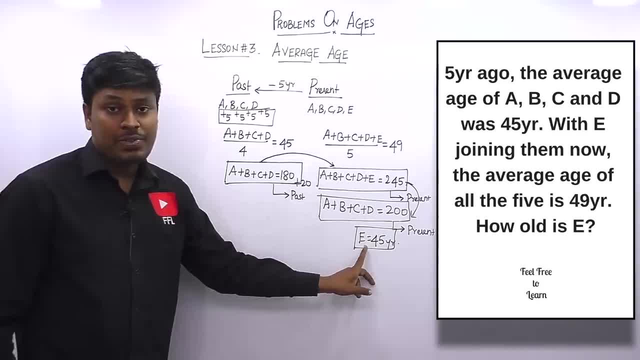 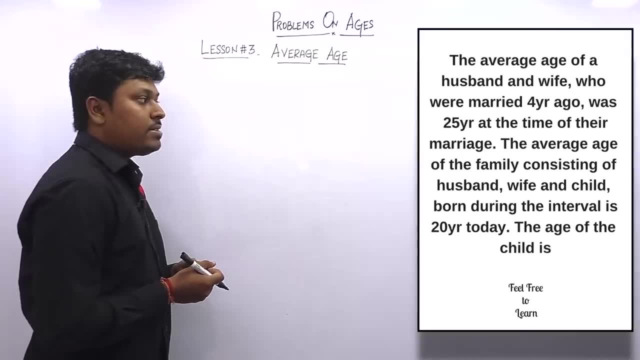 So we can say 245 minus 200 will be the age of the person E. So finally answer for question number 2 is 45 years. Question number 3.. The average age of husband and wife who were married 4 years ago was 25 years at the time of their marriage. 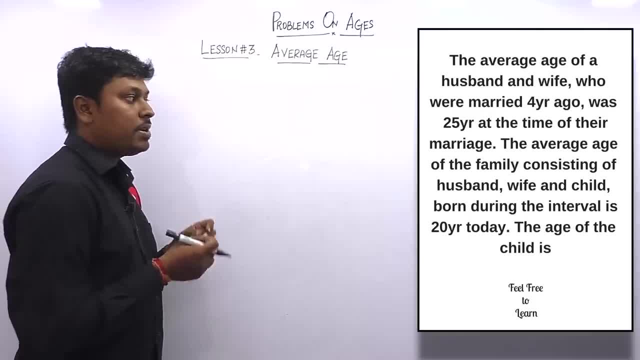 The average age of family consisting of husband, wife and child born during the interval 20 years. today, The age of the child is? This question is interesting because- first point, again, they are talking about the past, At the time of a marriage, that is, 4 years ago. 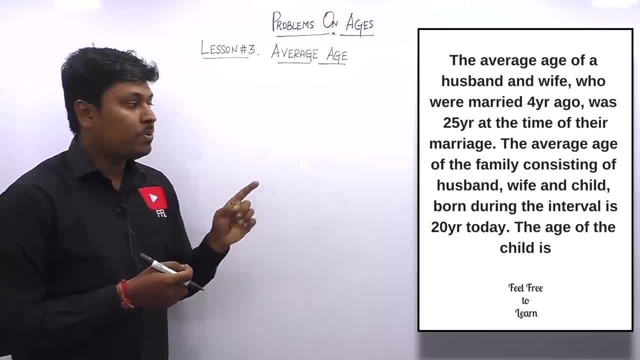 So they are talking about the past, where the average age of husband and wife is given, that is, 25 years. So between the time interval between 4 years. now they are talking about the present. Now the average age of father, mother and the child. 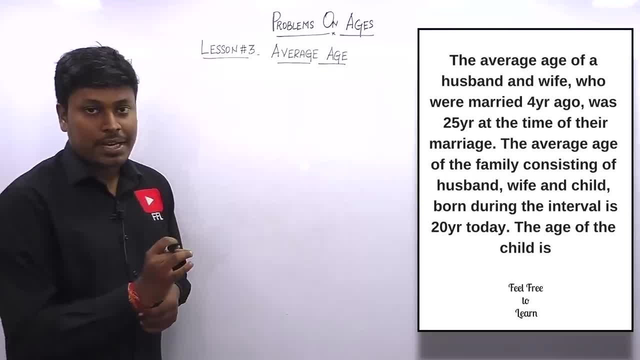 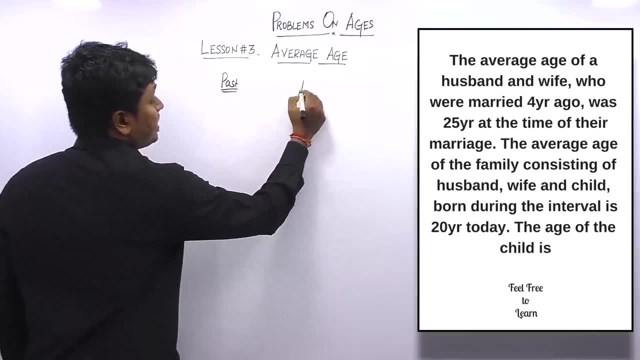 The average age is 20 years. So by using this data, our target- to find what is the age of the child. So listen here. In the first point They are talking about the past, So in the past. and the second point, they are talking about the present. 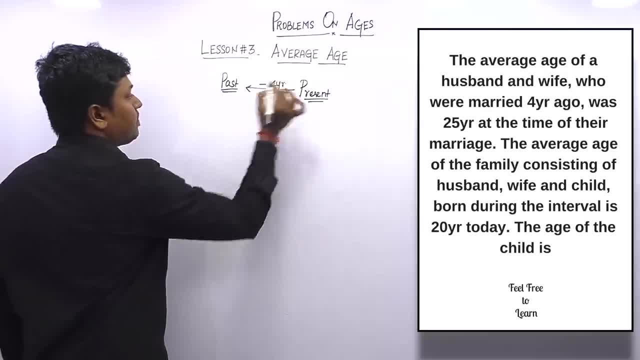 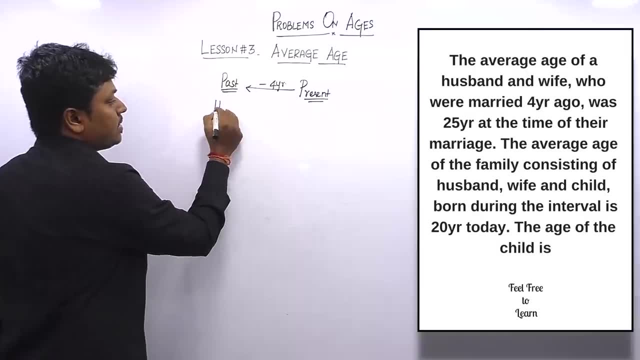 So from the present to the past, it's 4 years ago. So now what they are saying according to the first point, When the time of marriage, the time of marriage 4 years ago, where husband and wife average age is given, that is, 25.. 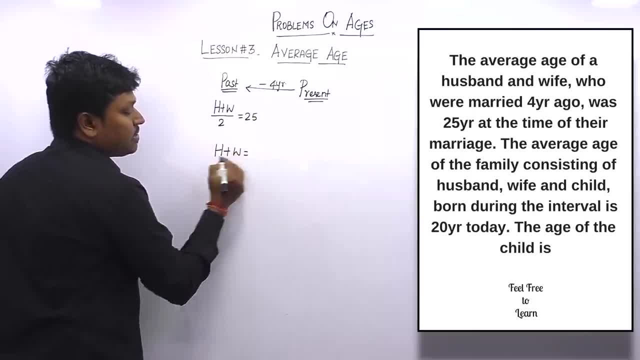 So we can say, at the time of marriage, some of their ages of husband and wife will be 50. So remember that This is the Equation that we framed for past. Most important right: Second: Now they are talking about a present where 3 person right. 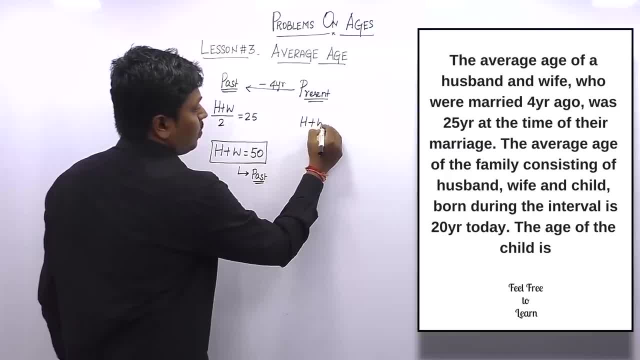 Husband, wife and a child. So husband, wife and a child. So divided by 3.. Now their ages. average age is 20 years, So we can say some of their ages of husband, wife and child will be 60 years. 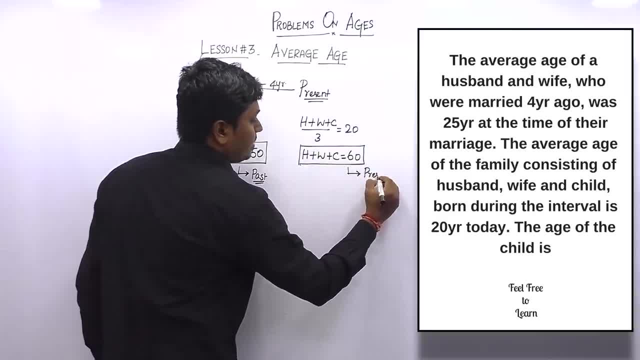 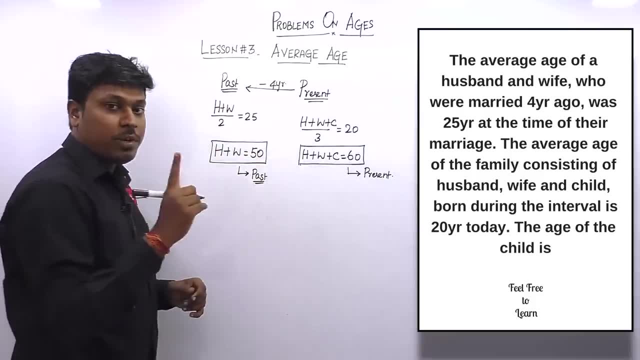 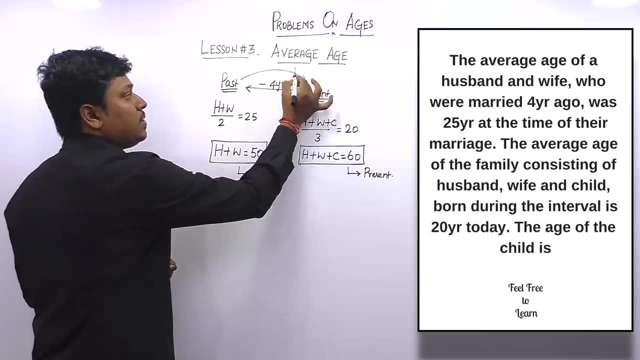 So this is the equation that we frame for present. So what you need to do, You should not directly Separate both the equation. that is completely wrong. So first step, what you need to do is you need to convert this equation, that is, past equation, to the present, right from the past to the present. you need to add 4.. 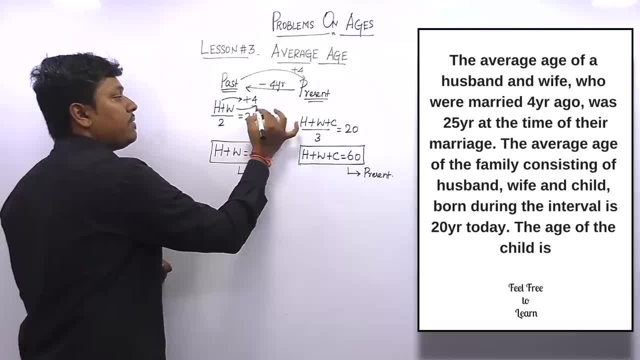 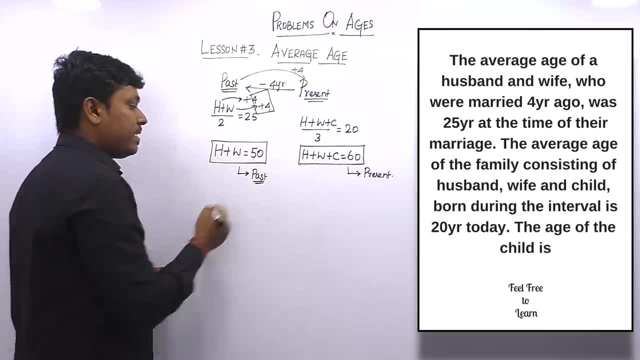 So in the age of husband, you need to add 4, and similarly wife, you need to add 4.. So, totally from past to the present, the total age of both the person is increased by 8, right? So once it is increased by 8- husband and wife- some of their ages will be 58. got it in the past, right. 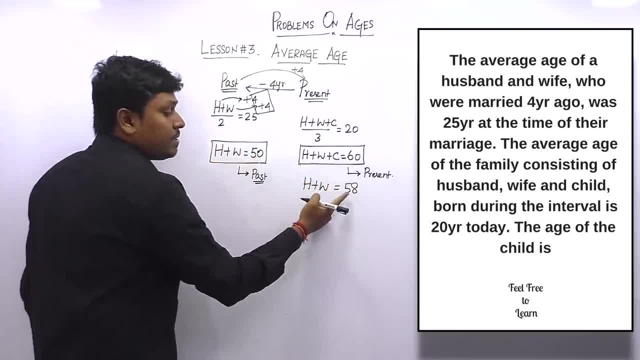 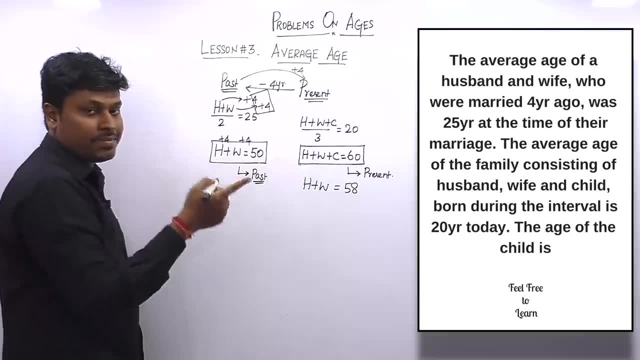 So we have 4 years back. some of their ages is 50. after 4 year The sum will be 50 because husband age is increased by 4. similarly wife age is increased by 4.. So total 8 years will be increased from the past to the present. 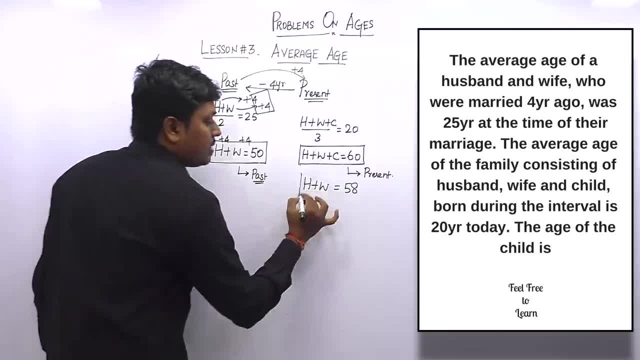 So we can say husband and wife, the total age will be 58. So this is the equation that we frame for the present. Now you can separate both the equation easily because husband and wife some will be 58. So instead of h and w, substitute 58 year. 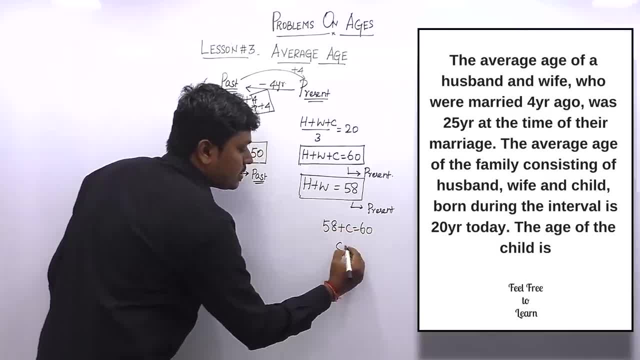 So 58 plus C is equal to 58.. So 58 plus C is equals to 58.. So 58 plus C is equals to 58.. 60. So C is equal to 2 years, which determines the child age will be 2 years. So finally answer for. 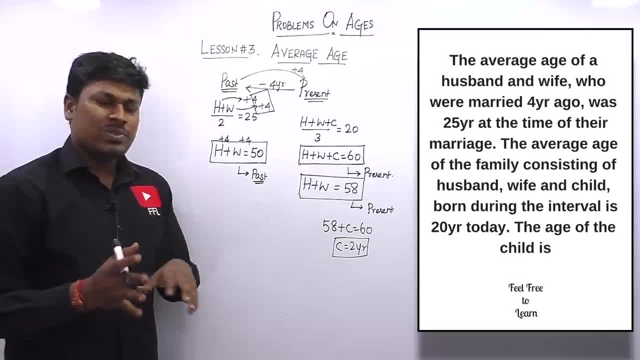 question number 3, where the age of the child is 2 years. So remember that if you are a beginner, try to solve like this. If you are an expert in problems on ages, according to me you can directly solve this question by using a shortcut or otherwise by using an options. But beginners, 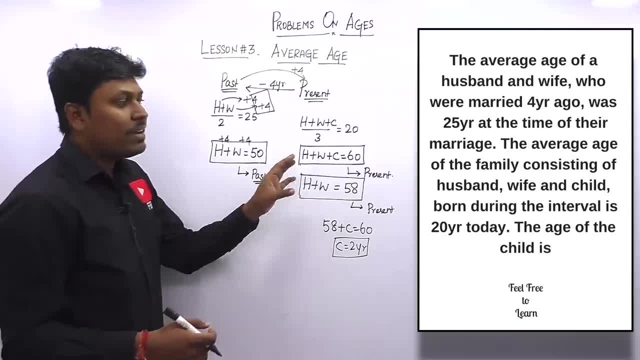 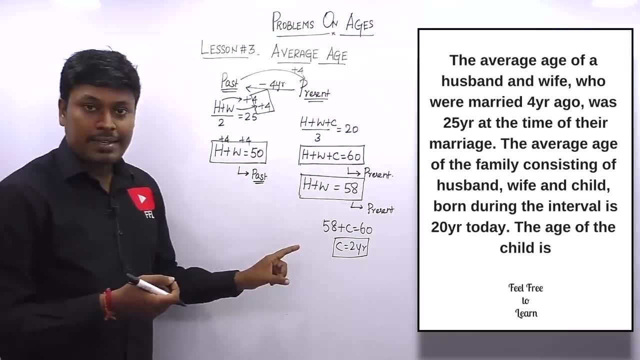 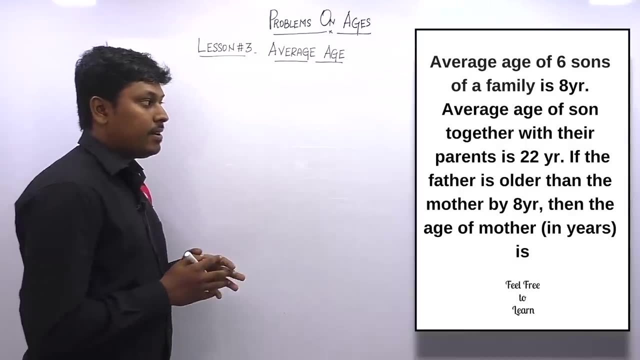 try to solve like a traditional method, only after solving 20 or 30 question, you too can able to solve the question in shortcuts, right? So finally, answer for question number 3, where the child age is 2 years. Question number 4.. Average age of 6 son of a family is 8 years. Average age of son together: 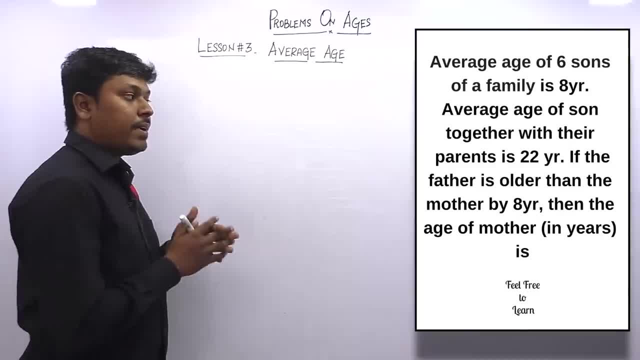 with their parents is 22 years. If the father is older than mother by 8 years, then the age of the mother in years. So according to this question, I would target to find what is the age of a mother and remember that in this question they are not talking about the past. 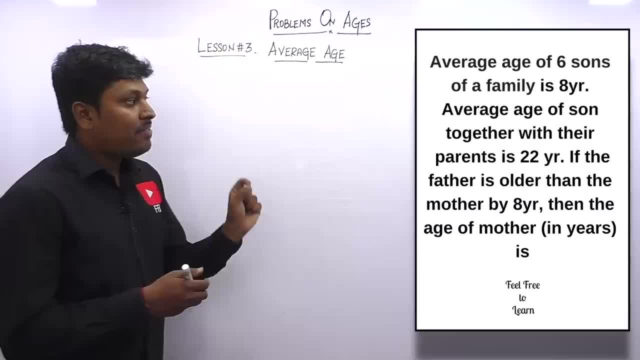 future, etc. They are just completely. they are talking about a present Average age of 6 son of a family is 8 years and similarly 6 son plus their family members, their average is 22 years. And last point, they have given a small note that where the father age is 8 years older than the mother, 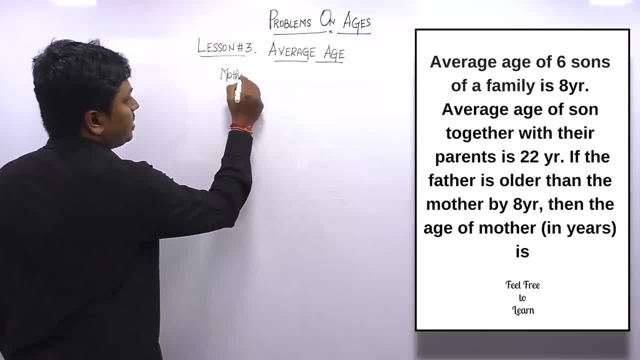 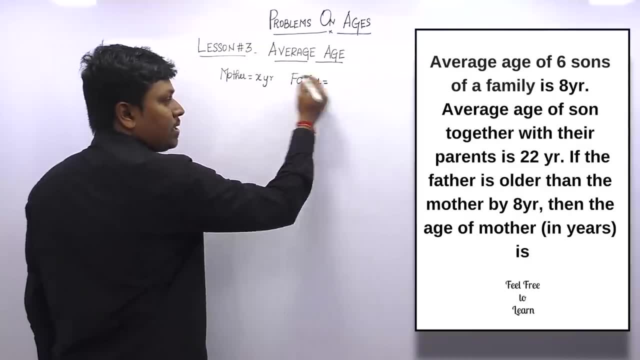 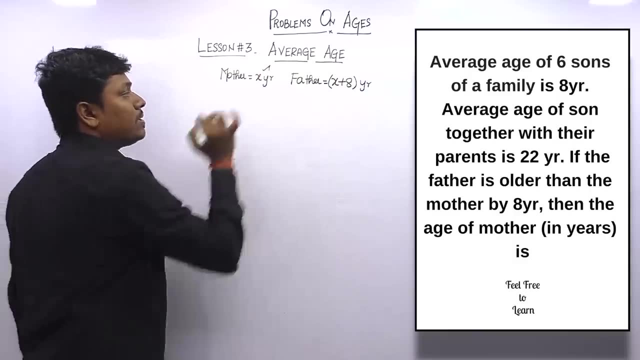 So let me do one thing. we can assume mother age as x, So mother is equals to x years. Then what about the father age? So father age, because 8 years older than mother, So we can say x is 8- will be the age of the father. But according to the question, our target to find what is the age. 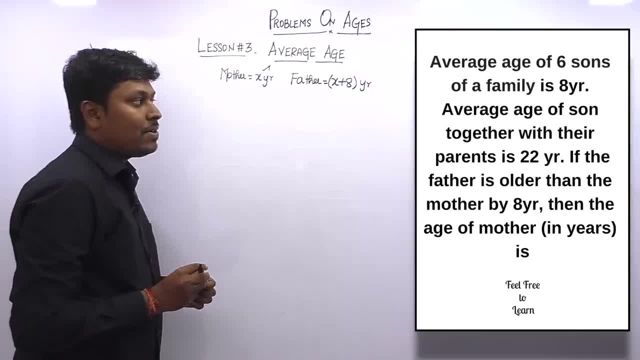 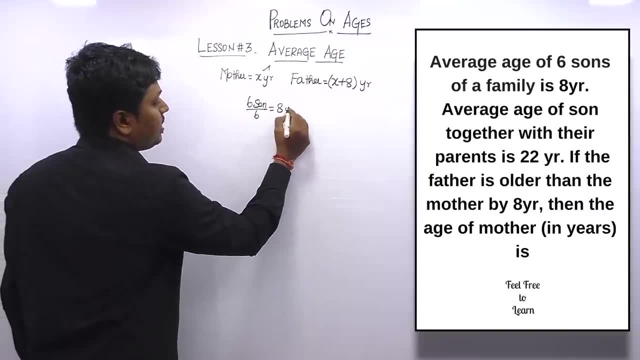 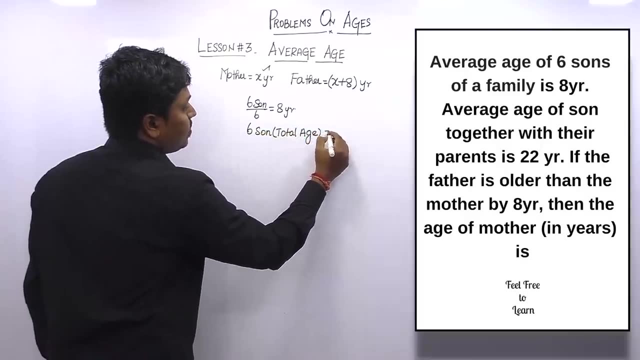 of the mother. So first point: average age of 6 son of a family is 8 years. So we can say sum of observation that is 6 son So divided by 6 is equal to 8 years. So 6 son total age is equals to. 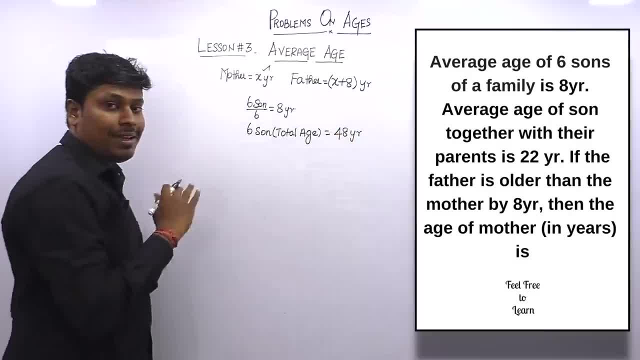 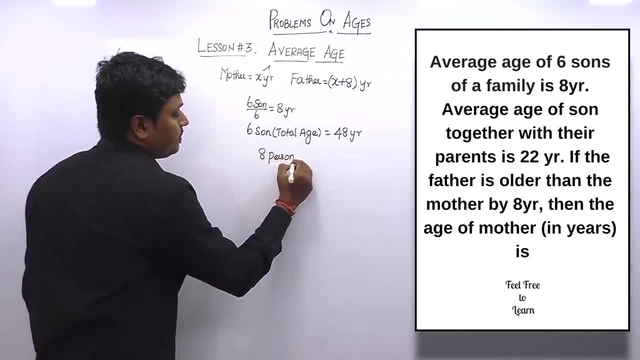 8, 6 years or 48 years. So sum of their ages of total, all the 6 son will be 48. In the second point, average age of son together with their parents. So totally 6 plus 2 person, that is 8 person. So 8 person divided by 8 and now they are saying the average is 22.. So 8 person. So this 8 person includes 6 son and a mother and a father. 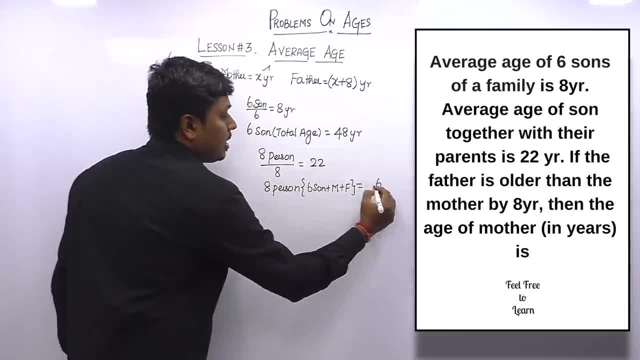 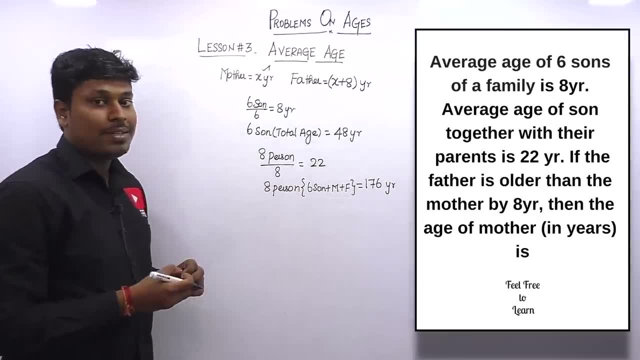 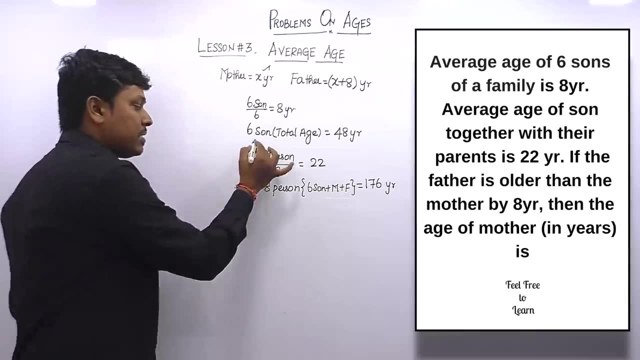 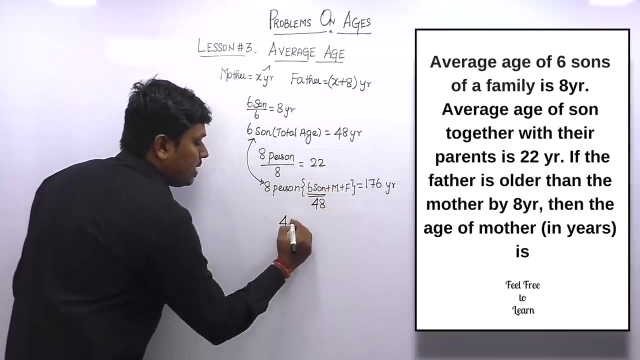 So is equal to 22 into 8 to 16.. Reminder will be 116, 17, 176 years. So total family member: some of their ages will be 176.. I think once you subtract both the value, you will get an answer that is father and mother alone. I am going to subtract both the equation in terms of 6, and here you can directly substitute this 48.. So 48 plus a mother and father will be 176. 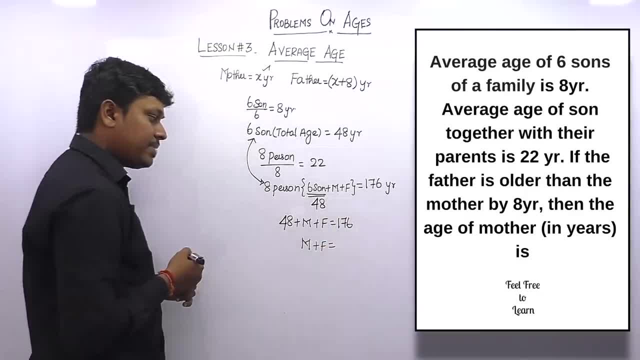 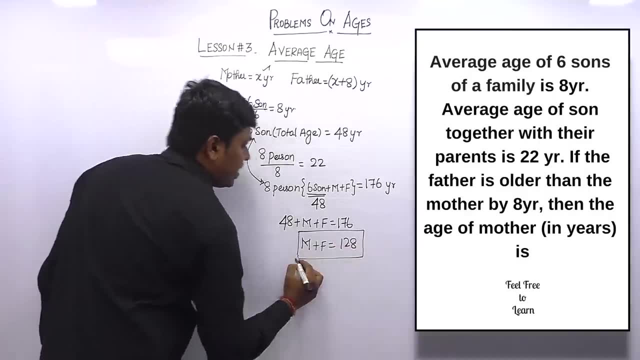 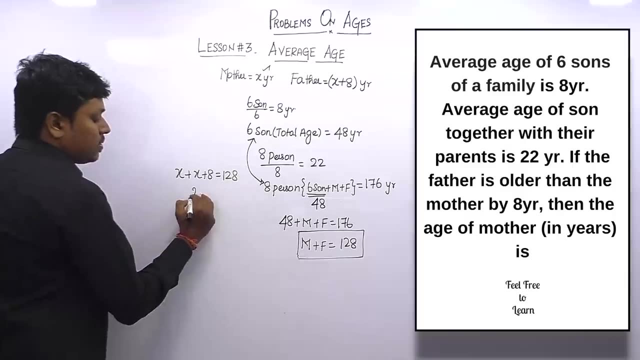 So mother and father age will be 176 minus 48 will be 128.. So we already assumed that mother's age will be x years, So x and the father will be x plus 8 is equal to 128.. So 2x is equal to 120.. So x is equal to 60. 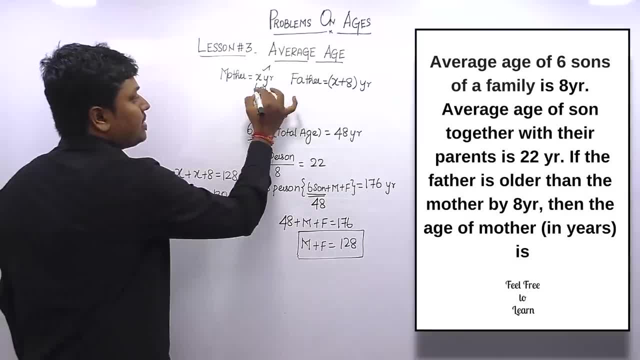 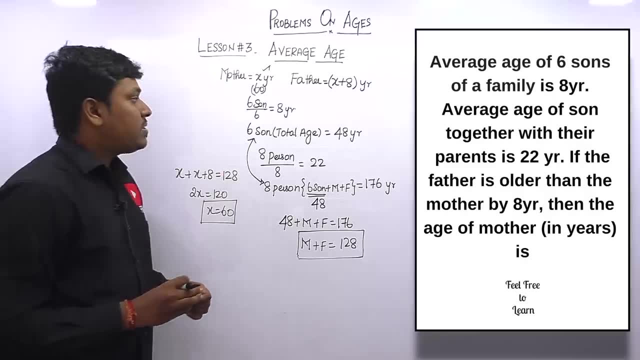 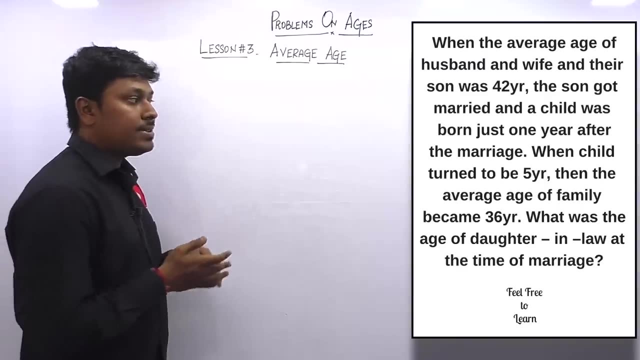 So finally we can say that mother age will be 60 years and the father age will be 68 years. So interesting question. So answer for this question number 4.. Age of a mother is 60 years. Last 5th question: When the average age of husband, wife and their son was 42 years, the son got married and the child was born just 1 year after the marriage. 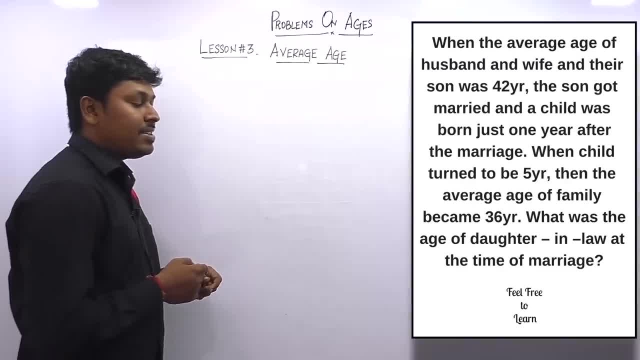 When the child turned to be 5 years, then the average age of family become 36 years. What was the age of daughter-in-law at the time of a marriage? Interesting question, and this was the question. It was a memory based equation of an SSE exam. 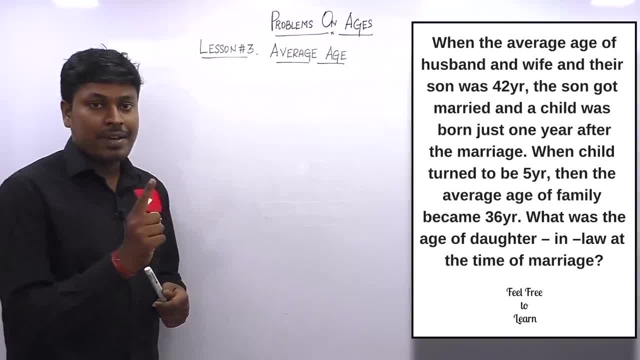 So listen here, They have given two average values. The first average value is father, mother and the son before marriage. They have given an average And the last value that is 36, it was given after 6 years, which is most important. Listen carefully. A son got married after 1 year. a child born. 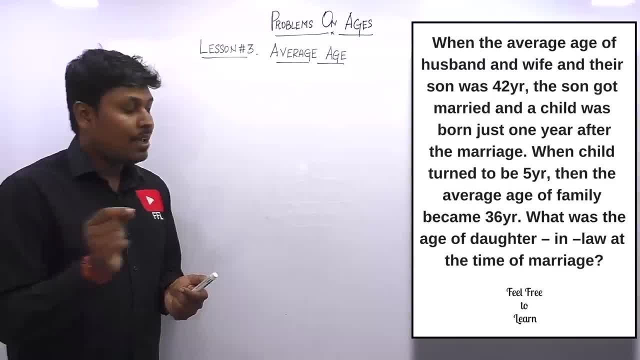 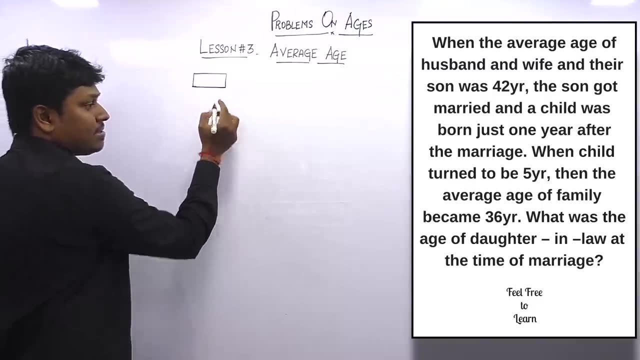 And the last value, that is 66 on average, is mother May be. in the worst case scenario, the son got married after 5 years. After 5 years, the child age became 5 years and average is 36 of the family. So by using the data we can find the age of daughter-in-law. 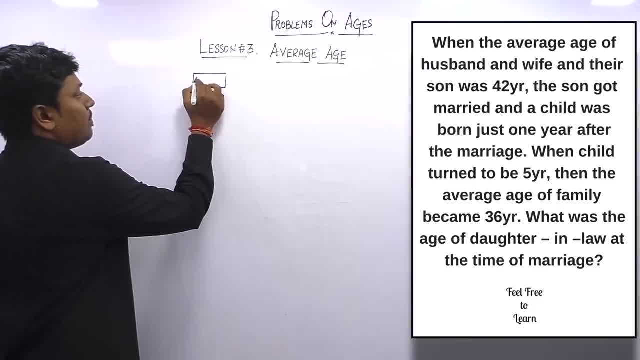 So let me submit something as my reference. Initially, they have given an average age: How much? 42 years. That is for a mother and a father and son, And then the son got married. Subscribe to our YouTube channel for new videos. 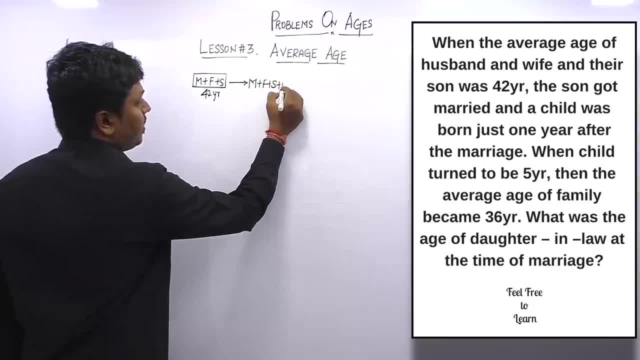 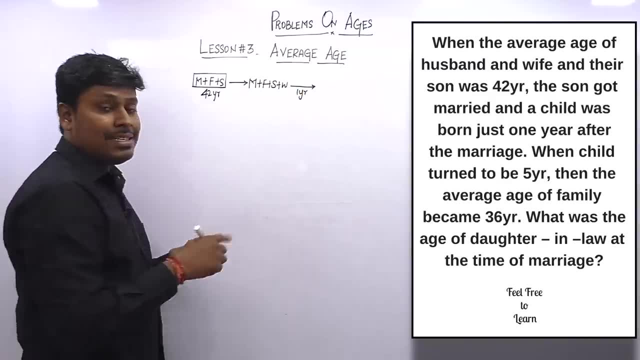 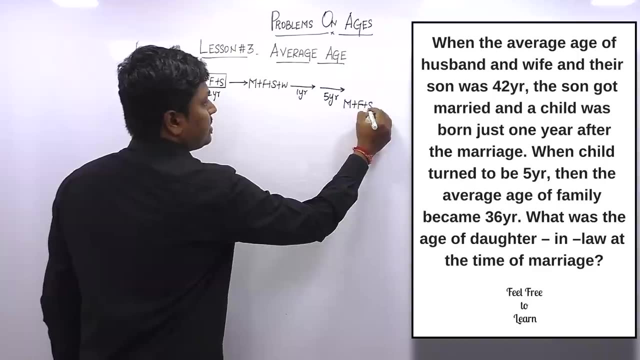 so mother, father, son and wife right after one year of marriage, so child born, and they have given that when child turned to five years, right, and another five years the average is given. that is mother, father, son, wife, which is daughter-in-law, then son, that is the child right, so let me keep it. 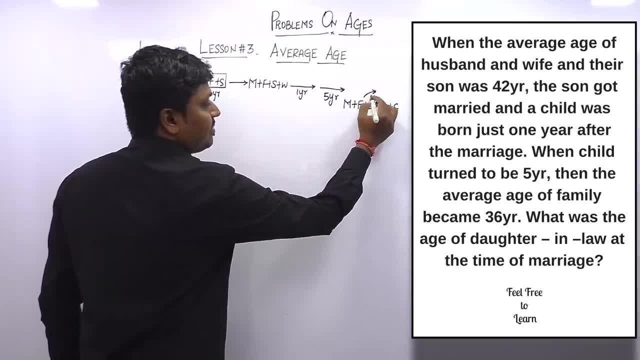 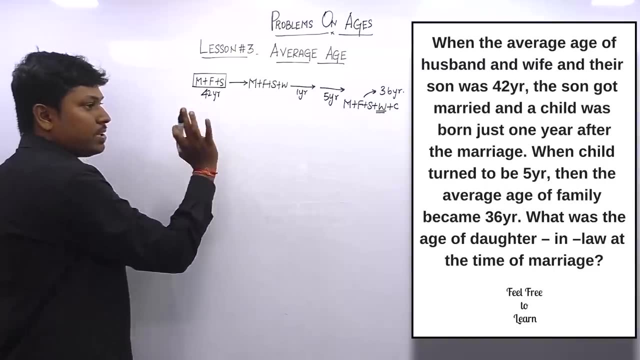 as c, so child, their average is given that is 36 years. very interesting question. so using this data, our target, to find the age of this daughter-in-law right that the son's wife is called as a daughter in law. so let me do one thing. first of all, we can find what is sum of their ages of all the three. 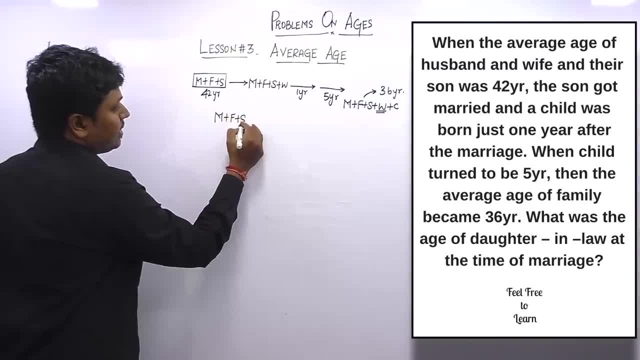 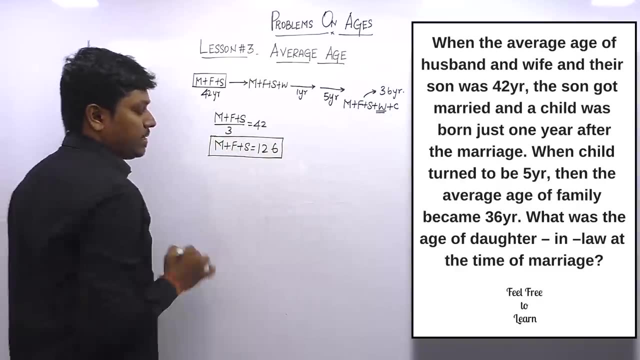 person, right? so mother, father and the son. so divided by 3 is equals to 42 year. so mother, father and the son, so total sum of their total ages will be four, three, two, six, one twenty six. so one twenty six will be the total age. so listen carefully what they are saying is. and then son got married right after one year child. 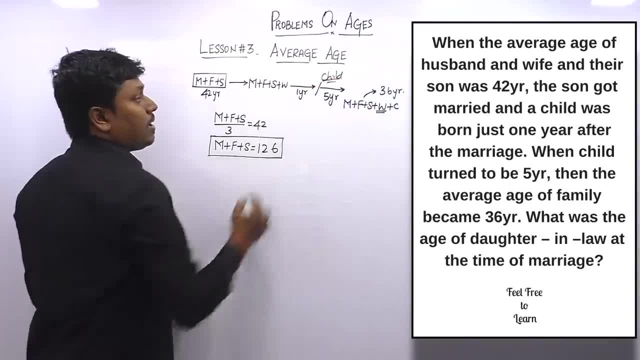 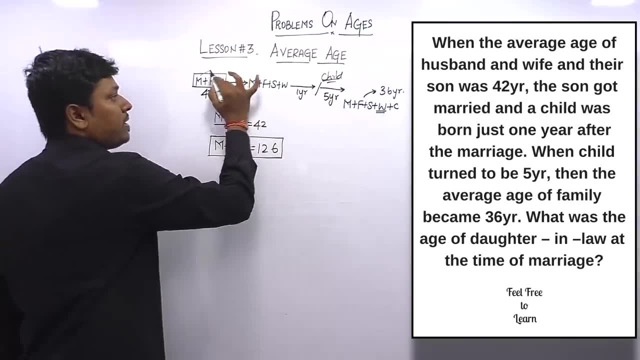 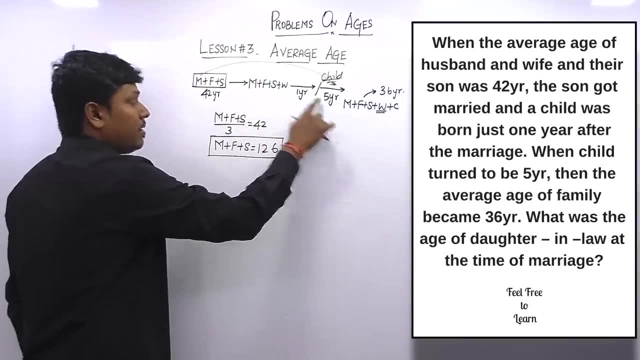 born right. so this time the child born, and again what they are saying. after the child turned to five year, the average age is given. listen carefully. so from this point to this point, right to this future, what you need to do? you need to add one year and another five year, so totally. 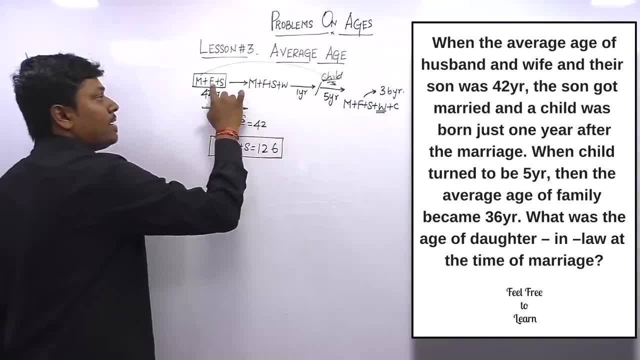 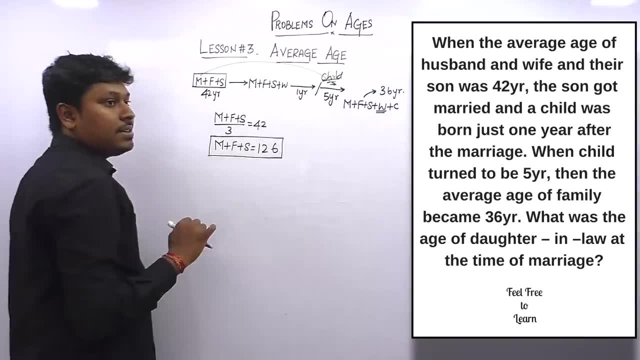 nothing happens in this age, right? so if you look now at the little star in the moving here, you will find a story on a kind of ratio, telling about what her mother is. but she's a very авать. eight is heroes, right? so if you observe what she says is that generally father is six. 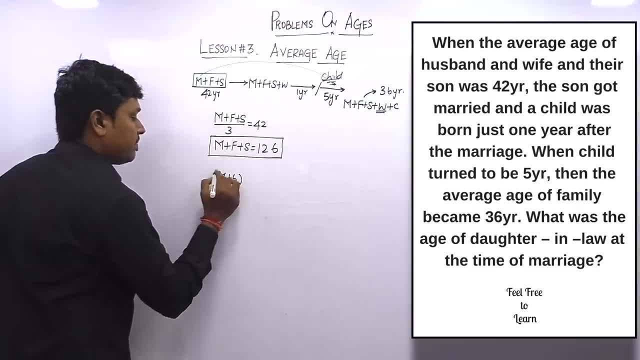 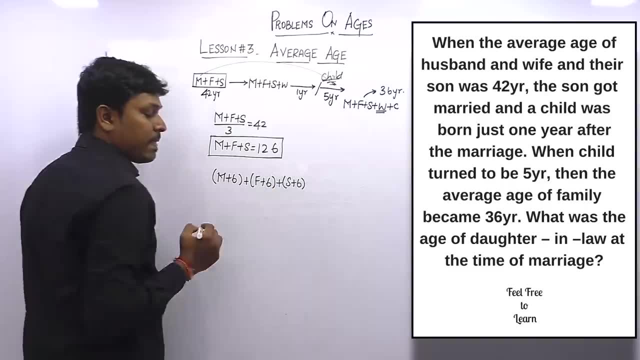 years, but father is younger but she is having six years in the two years. similarly, motherage is increased by six year. similarly, father age is increased by six year and the son age is increased by six year and where the wife age is increased by six year but the child age. 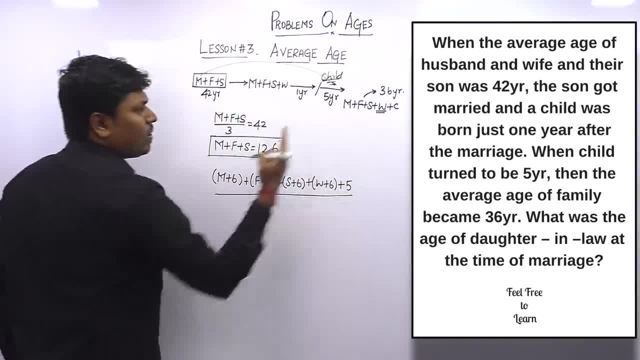 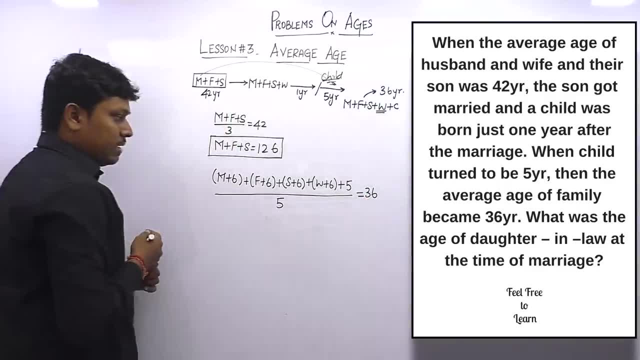 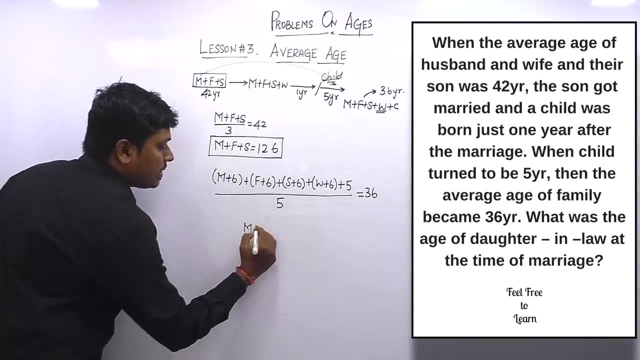 the same, that is 5. so divided by now they have given how much power: 1, 2, 3, 4, 5. totally there are five person and the average age is given that is 36. now I think six, fours are 24, so 24 plus 5 will be 29. so we can say: mother, father, son. 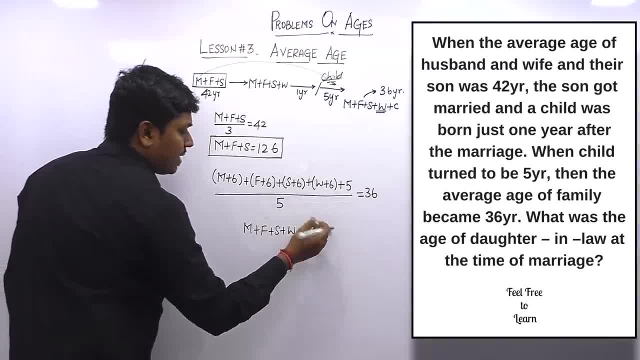 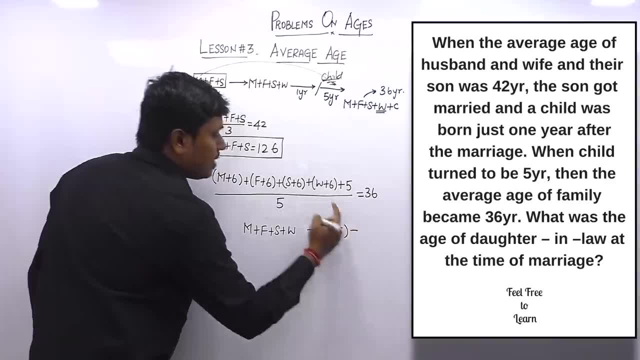 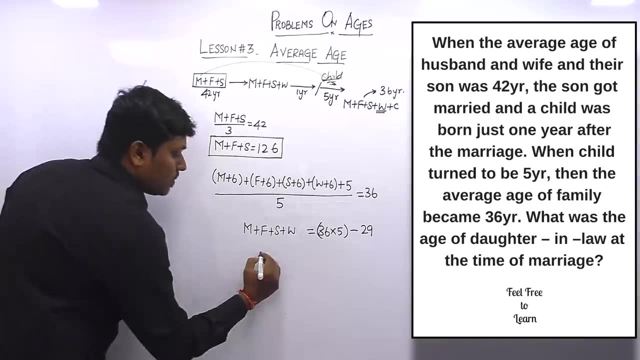 wife and a child, right so child which we have taken as five year directly. so all the four person as equals to 36 into 5. so minus of six fours are 24. 24 plus 5 will be 29, so minus of 29. so M plus F plus S plus W was equals to six fives.